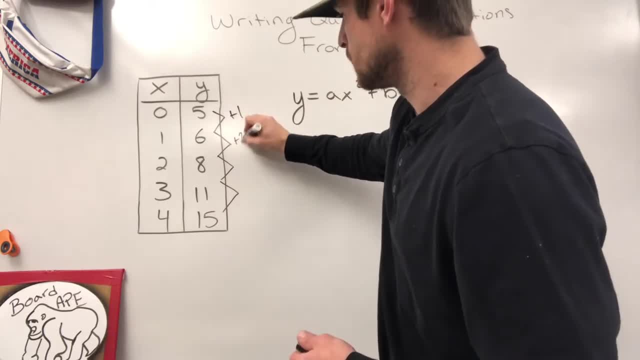 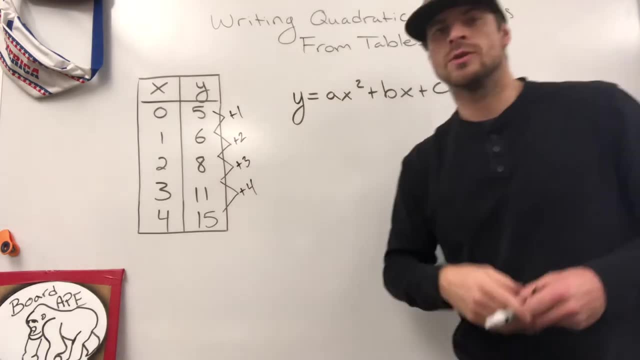 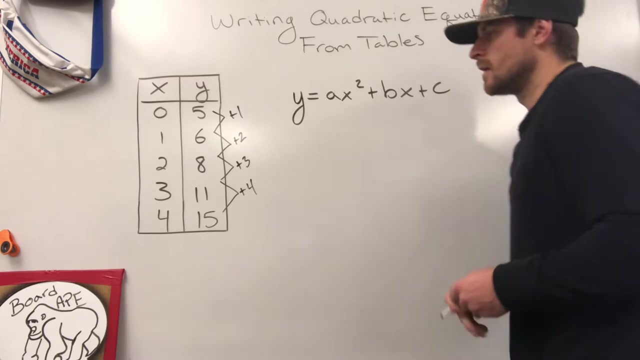 is constant. We're going up one, up two, up three and up four. What we're dealing here with is a quadratic. All right, what you need to do in order to find out the equation for a quadratic is you need to determine what the a, the b and the c values are. Okay, I'm going to 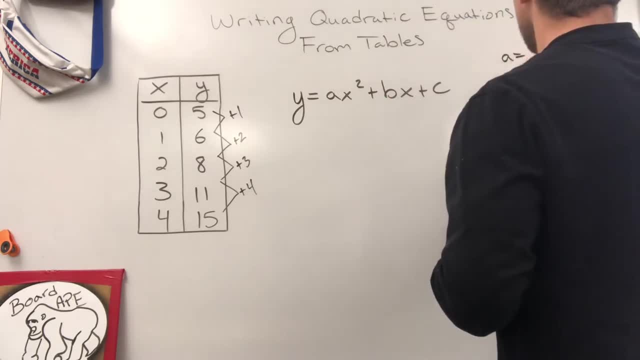 tell you how to find each one of those. So we're going to need to find a, we're going to need to find b and we're going to need to find c. I'll write those off And we'll track them as we find them. A is found, okay, a is going to be found from your second. 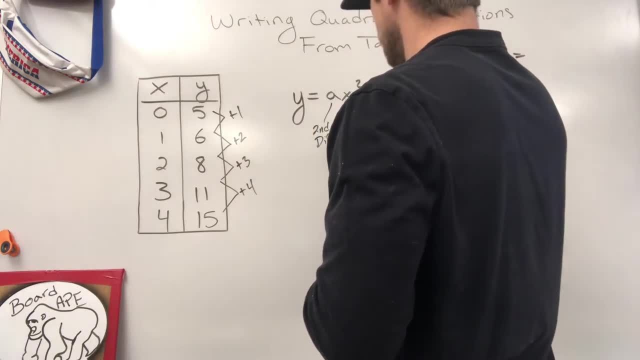 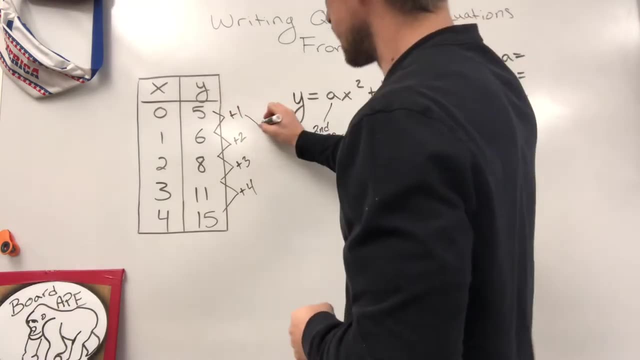 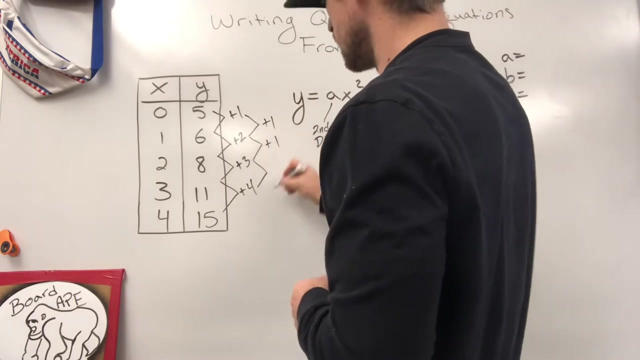 difference, your second difference, And what that means is: we look here, we do not have a constant rate of change on our change in y, so we go to our second difference. Between those numbers, what's happening? One to two plus one, two to three plus one. 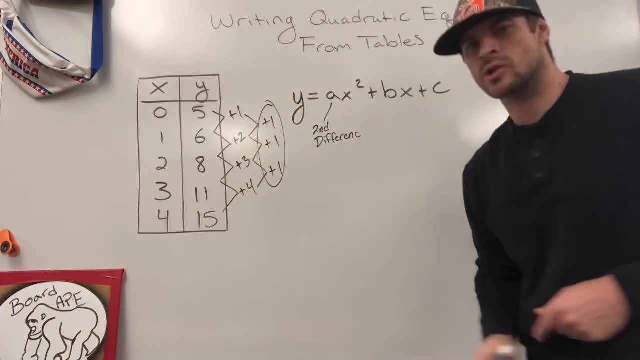 three to four plus one. I like what I'm seeing. I'm going to circle it. That's going to help me. I'm going to circle it. I'm going to circle it. I'm going to circle it. I'm going to circle. 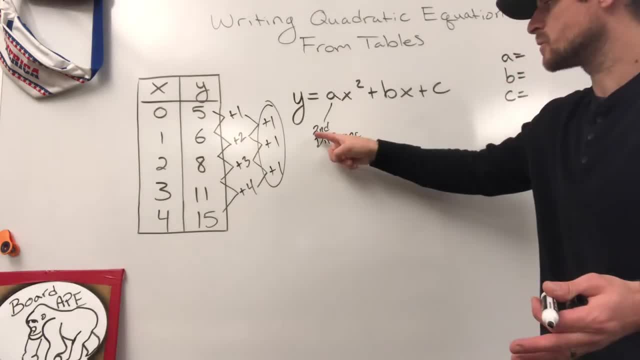 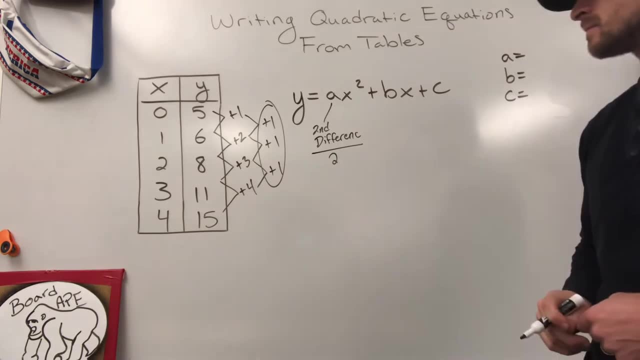 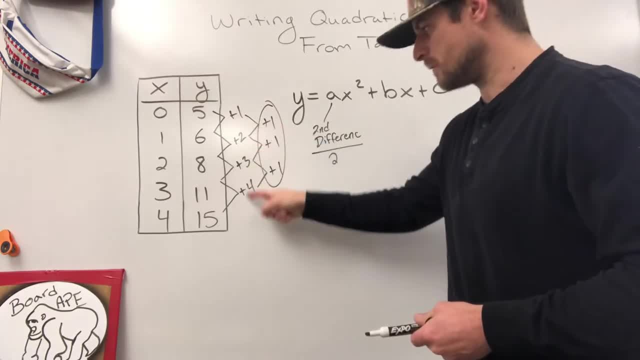 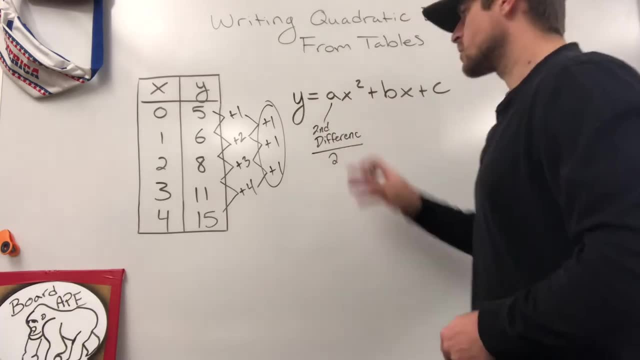 two. So I went my first difference one, two, three, four. Second difference: one, one, one. So I'm going to take one that's my top, or my numerator, to one over two. So I now know that a. 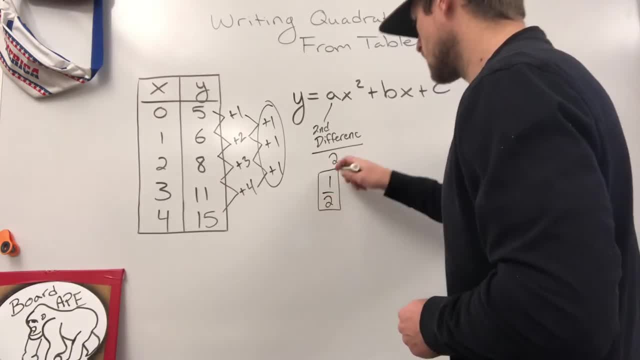 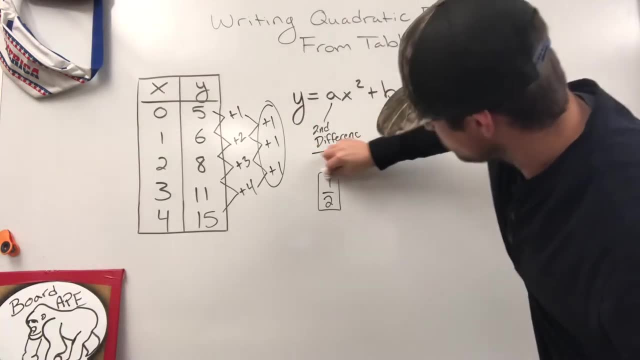 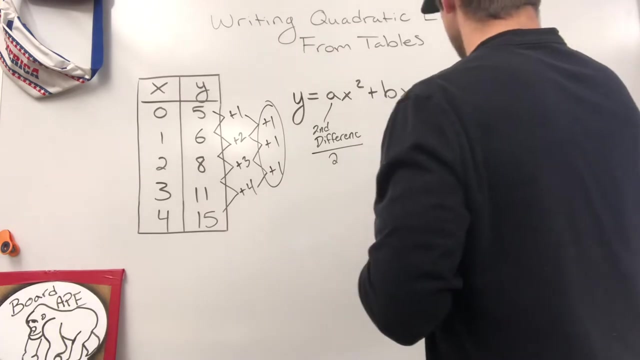 is one over two. I'm going to put that over here so I can keep track of it. A is 1 half. B is what we'll find last C, however, C is your 0 term When x is 0,. where are you at? 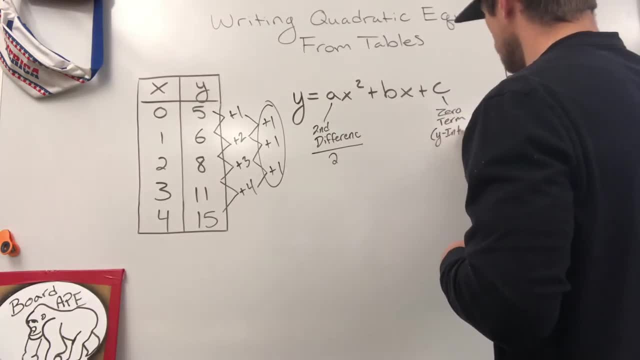 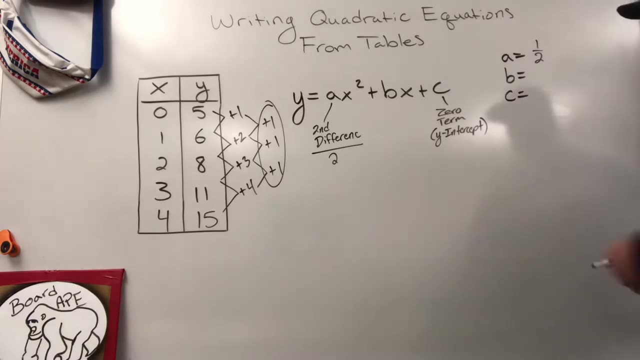 It's also known as the y-intercept. You probably know that from your linear equation unit back in algebra 1 or pre-algebra. So we have our starting point, our y-intercept. So we go to our table. Our 0 term is 5.. 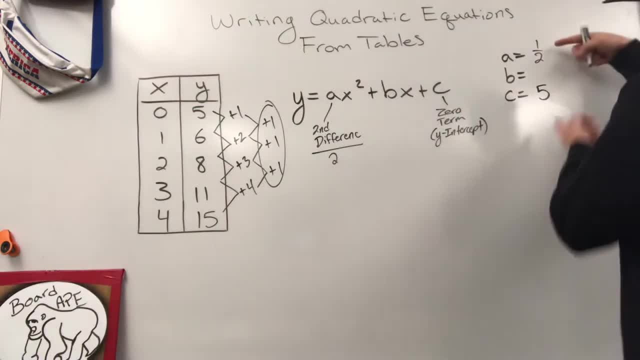 That's our starting value, So C is 5.. Hey, I've got two of the three parts that I need. The trickiest one to find, however, is B, And here we go Now. a lot of times, kids are stuck. 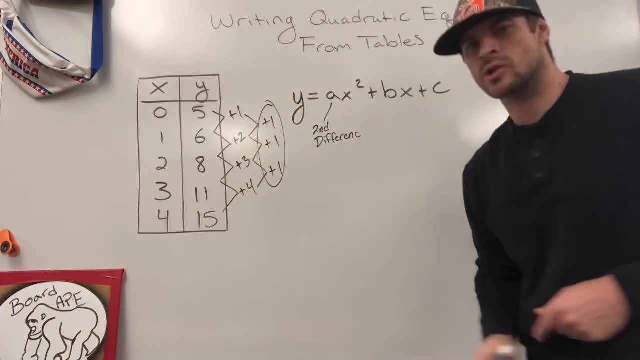 three to four plus one. I like what I'm seeing. I'm going to circle it. That's going to help me. I'm going to circle it. I'm going to circle it. I'm going to circle it. I'm going to circle. 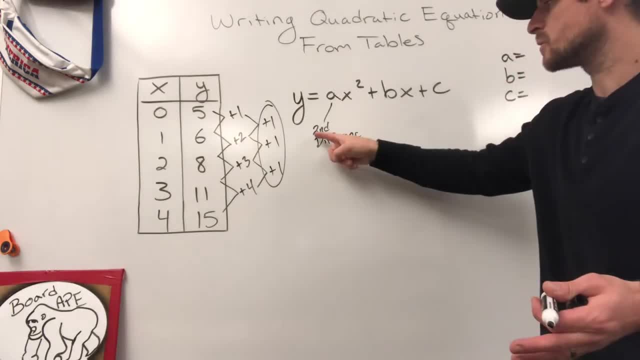 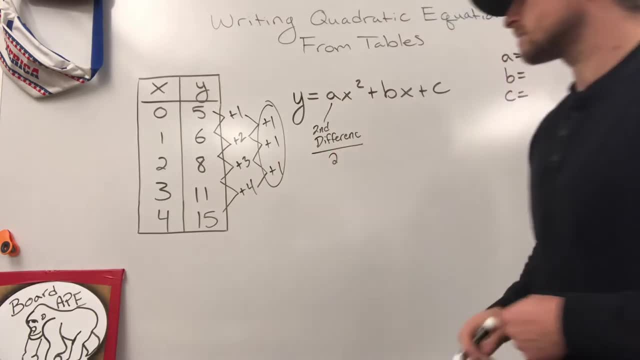 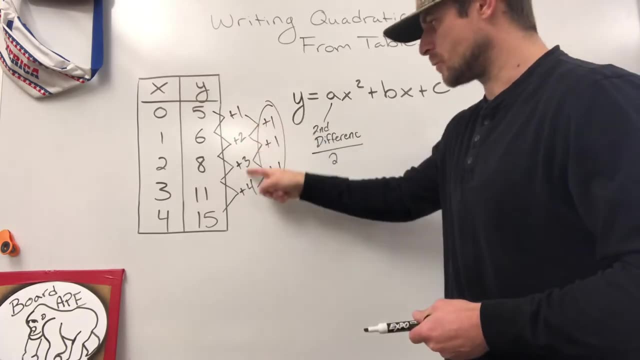 divided by two, Second difference divided by two. So I went: my first difference: one, two, three, four. Second difference: one, one, one. So I'm going to take one. that's my top or my numerator. 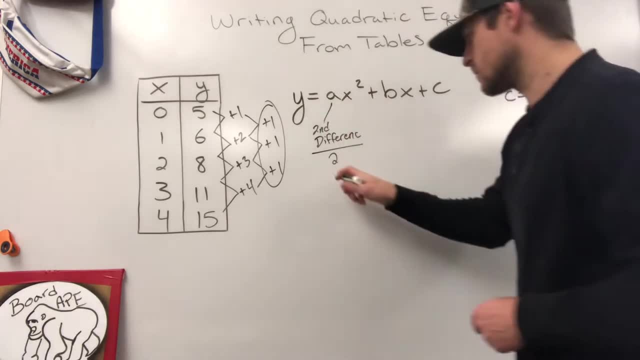 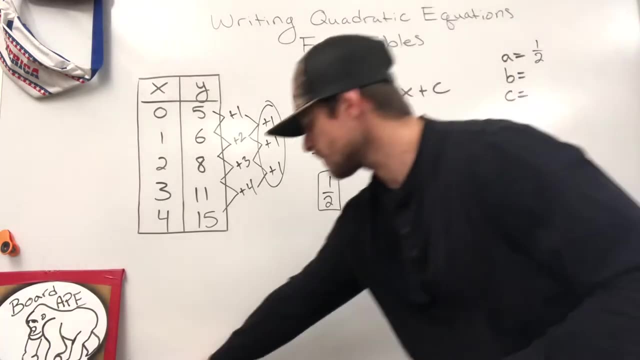 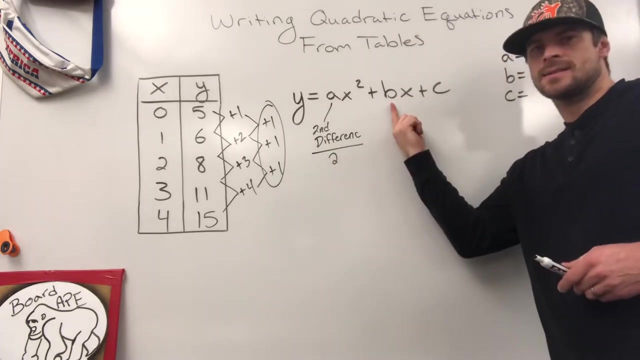 to one over two, So I now know that a is one over two. I'm going to put that over here so I can keep track of it. All right, a is one half. B is what we'll find last C. however, C is your zero term. 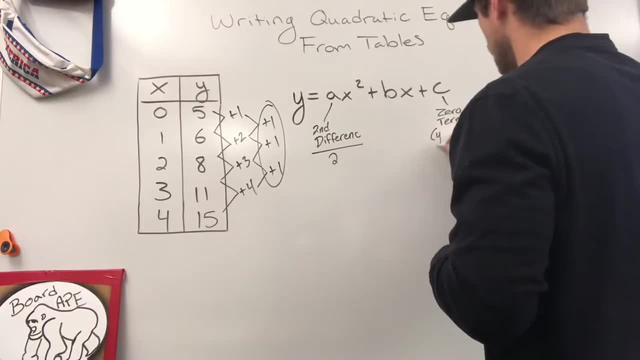 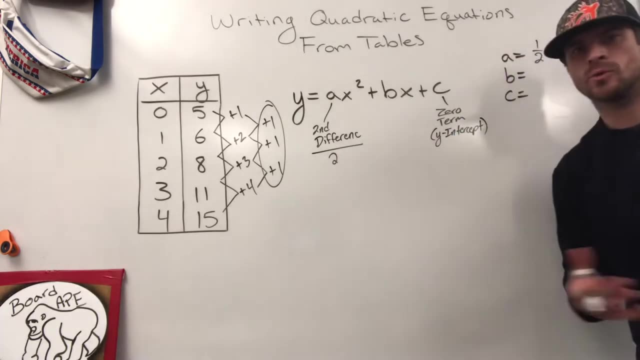 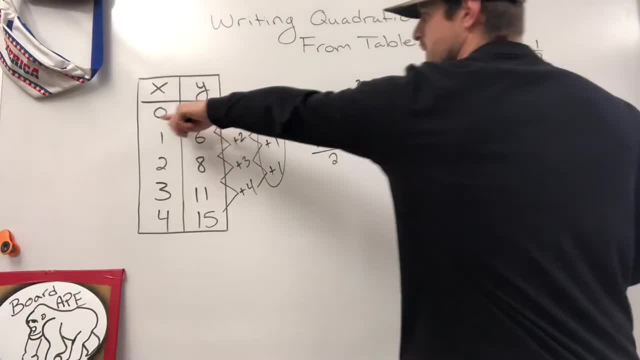 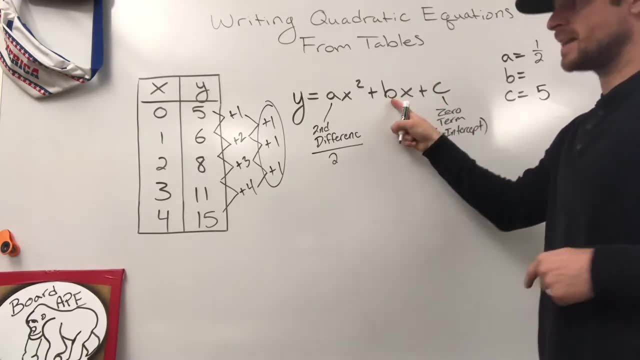 Our y-intercept. So we go to our table. Our zero term is five. That's our starting value, So C is five. Hey, I've got two of the three parts that I need, The trickiest one to find, however. 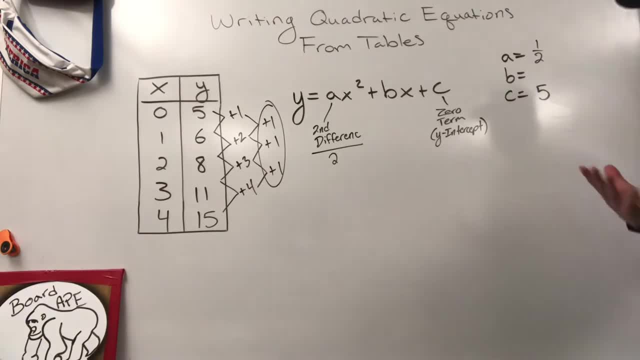 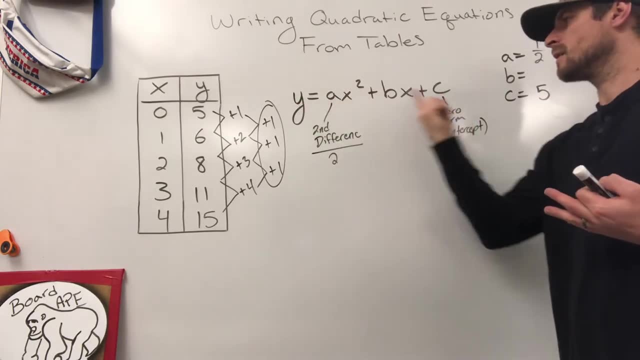 is B. and here we go. Now. a lot of times kids are stuck. They're like: well, just tell me how to find B. Well, I can't other than plugging in information here, here, here, here, here. 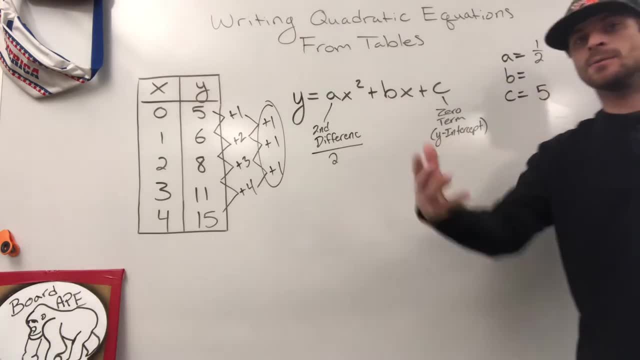 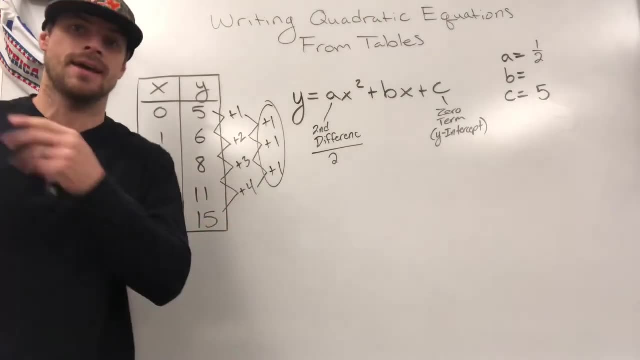 and leaving B to be the only variable left, and then we can solve. Remember back when you were solving for x all the time, You know you had to do the distributed problem, you had to do the property inverse operation- all that good stuff to get x by itself. Well, we're going to write a y. 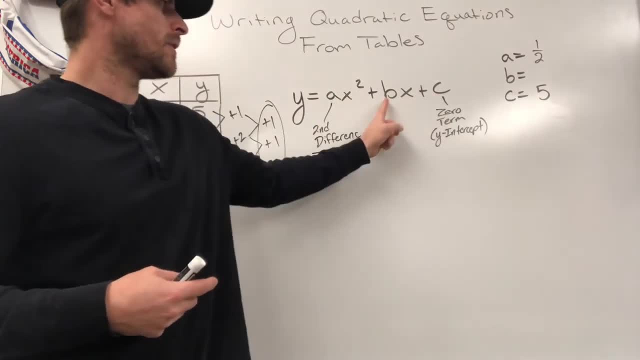 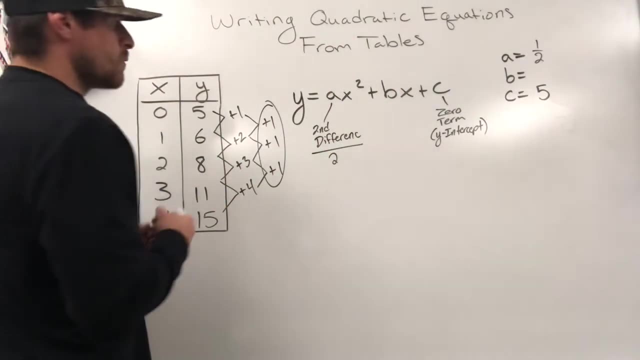 down, an a down, an x down, an x down and a c. The only variable left is going to be B, and then we'll just work downward to solve for it. All right, so let's write what we know. I know y. 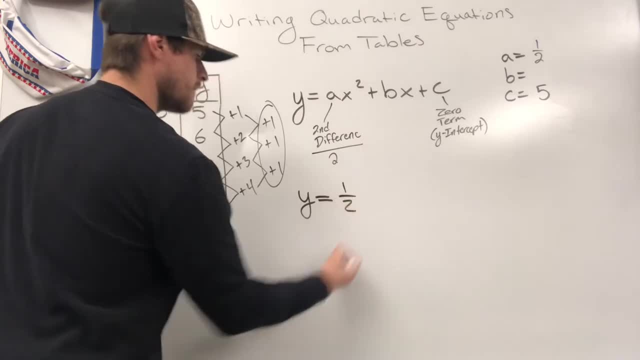 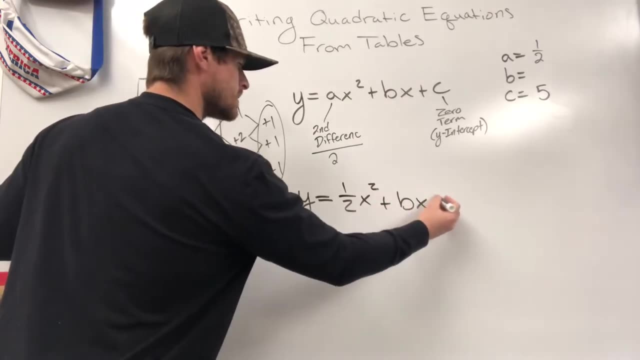 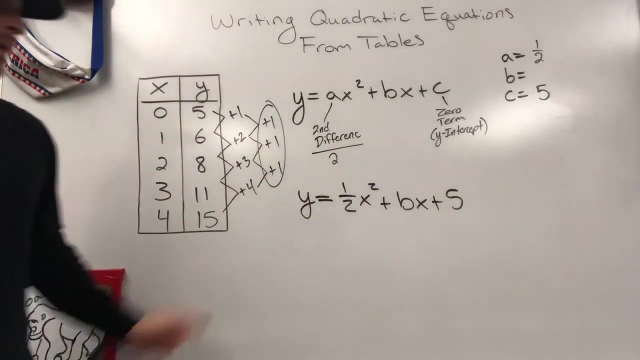 equals. I know a can be written as one half x squared plus B x plus five, because I changed the c to a five because I know it's my zero term. Well, this is all fine and dandy, except I'm still missing B, and the only way to get B is if I can. 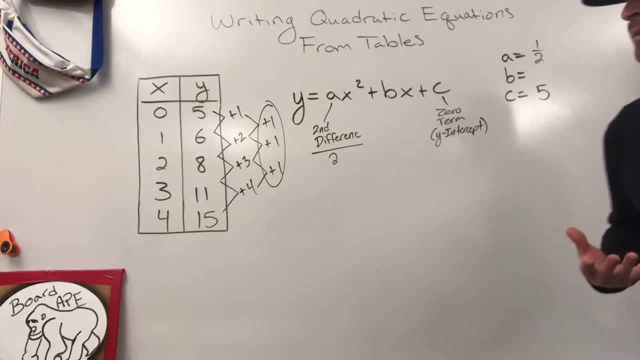 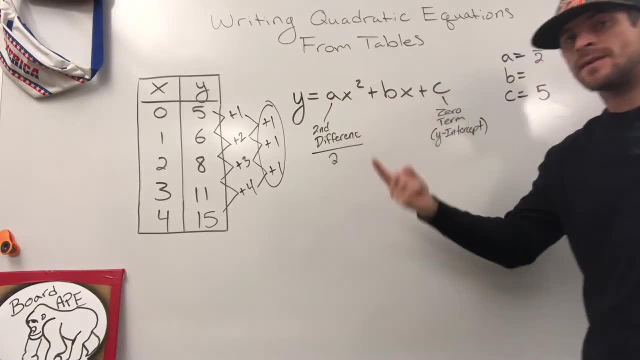 They're like: well, just tell me how to find B. Well, I can other than plugging in information here, here, here, here here, and leaving B to be the only variable left, And then we can solve. 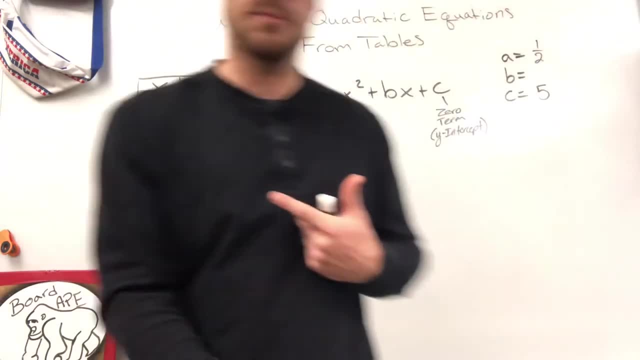 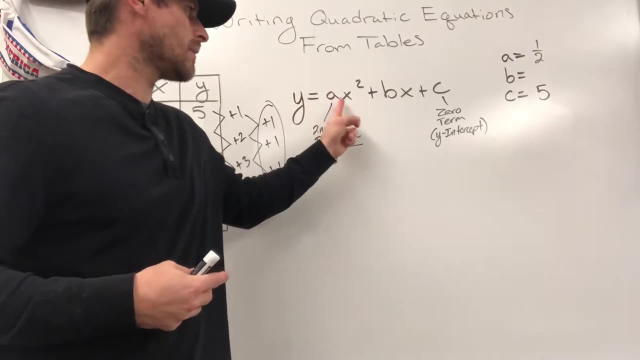 Remember back when you were solving for x. all the time You had to do this, You distributed property, inverse operation, all that good stuff to get x by itself. Well, we're going to write a y down, an a down, an x down. 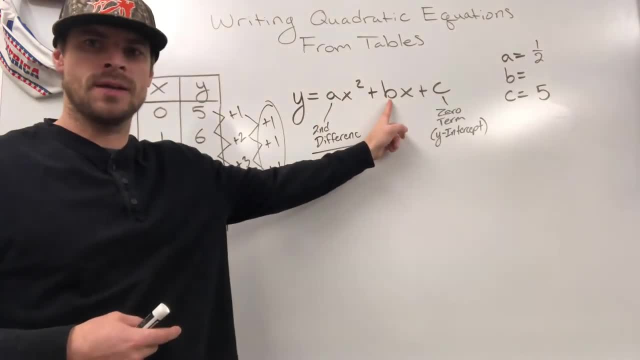 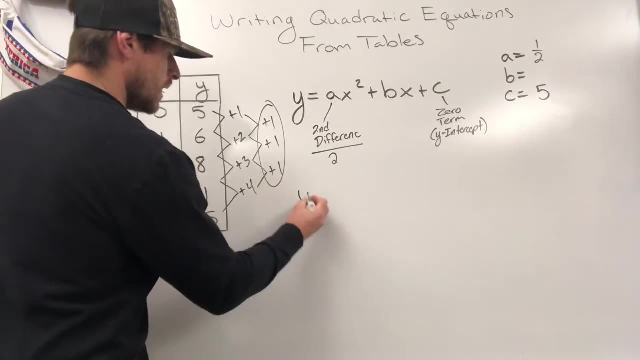 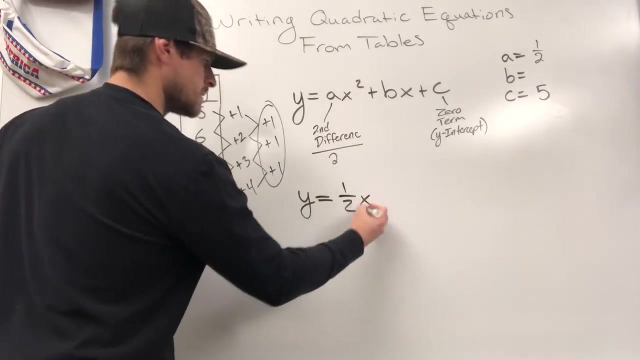 an, x down and a c, The only variable left is going to be B, And then we'll just work downward to solve for it. So let's write what we know. I know y equals. I know a can be written as 1 half x squared. 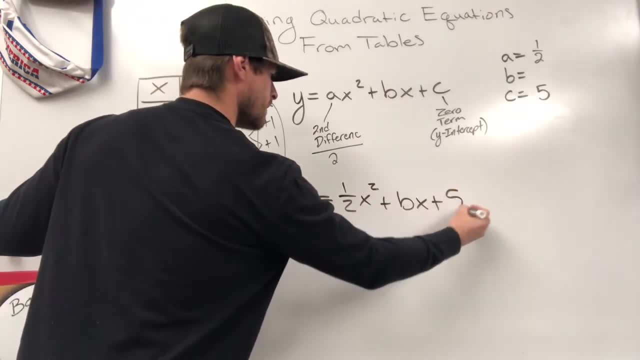 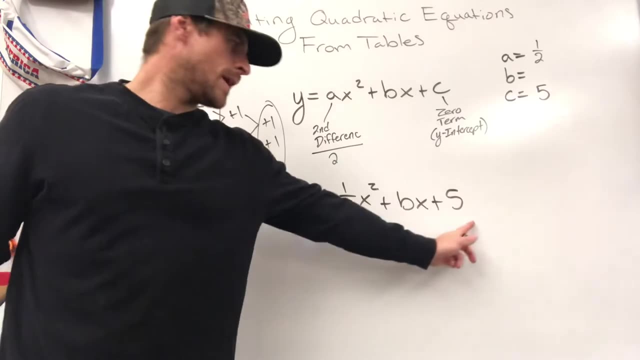 plus Bx Plus 5.. Because I changed the c to a 5, because I know it's my 0 term. Well, this is all fine and dandy, except I'm still missing B. And the only way to get B is if I can change that x to a number. 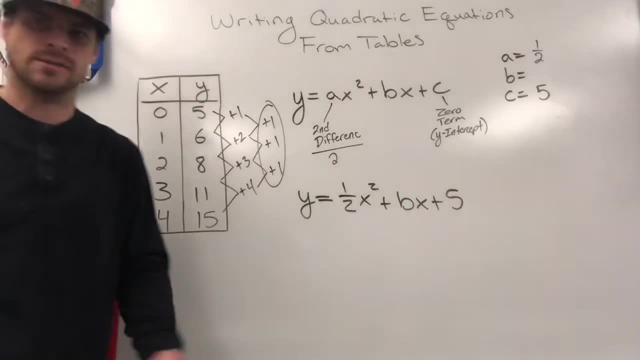 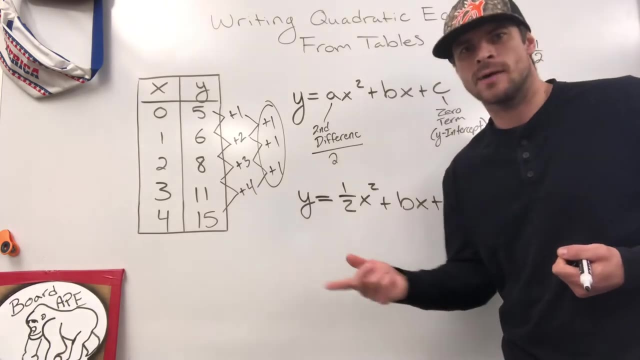 that x to a number and that y to a number. so I can start to simplify some things. Well, where in the world am I going to find some x values and some y values? Yeah, I was just blocking it. Look at that. 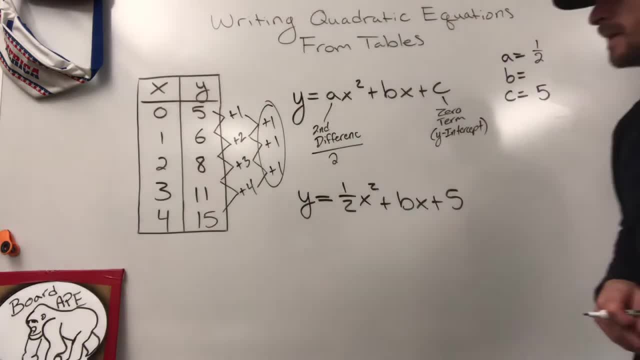 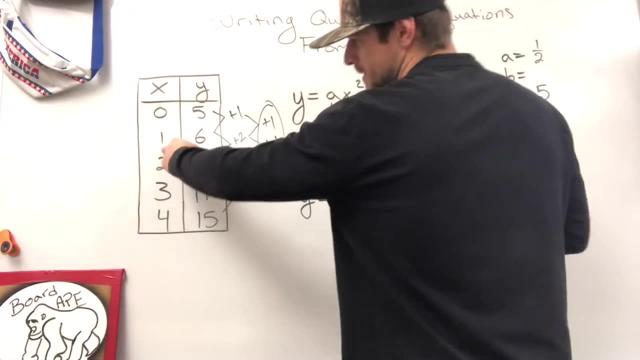 You've got a ton of possible numbers that you could put, Numbers that you could plug in there. Pick one and go with it. I recommend not using 0. So I always use the one that's closest to 0, because those are typically the lowest numbers. 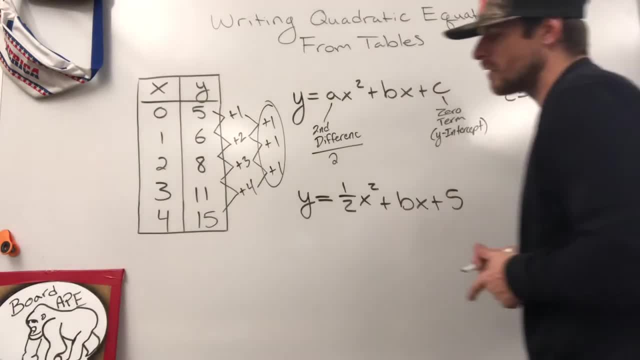 And small numbers are easy to work with. Come on, quit making your life hard. I've got kids that will always choose 4 and 15, or these big numbers, And I'm like you're just making your life more challenging. 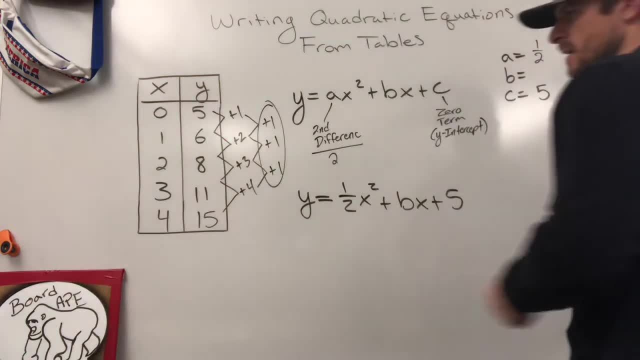 Pick the easiest two numbers you can find. 1 and 6 look great. 2 and 8 look great. Now I will tell you one thing right now: If I'm going to take something and scroll it, and I'm going to write it down, and I'm going to write it down, 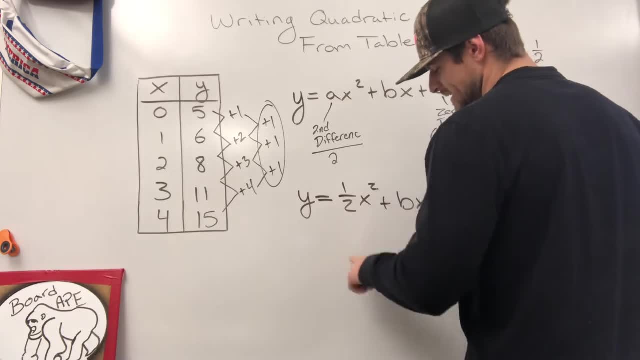 I'm going to write it down, and I'm going to write it down and I'm going to write it down and I'm going to write something and square it and then multiply it by a half. I'd like to get a whole number here, ideally. 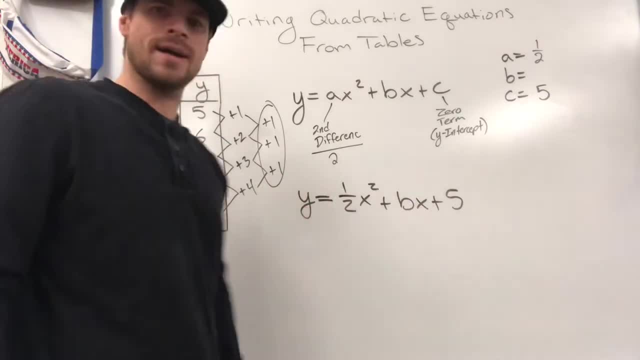 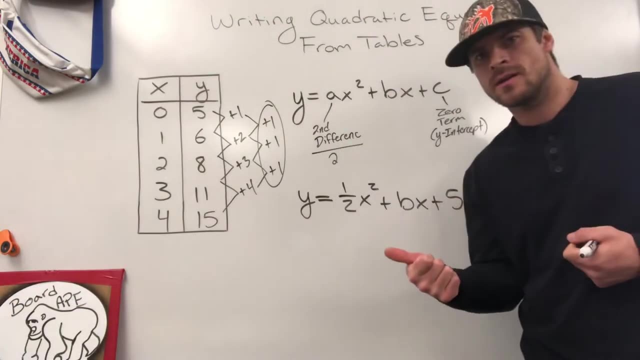 change that x to a number, that x to a number and that y to a number, so I can start to simplify some things. Well, where in the world am I going to find some x values and some y values? Yeah, I was just blocking it. Look at that. You've got a ton of possible numbers that you can plug in. 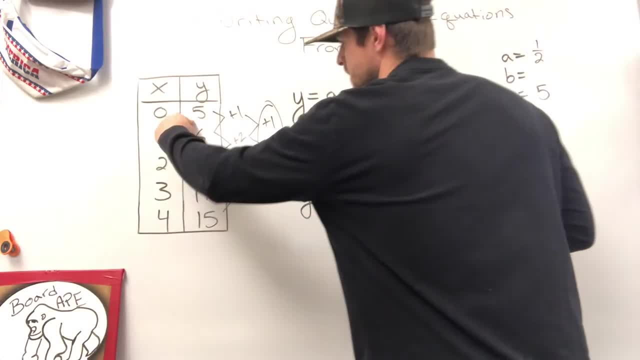 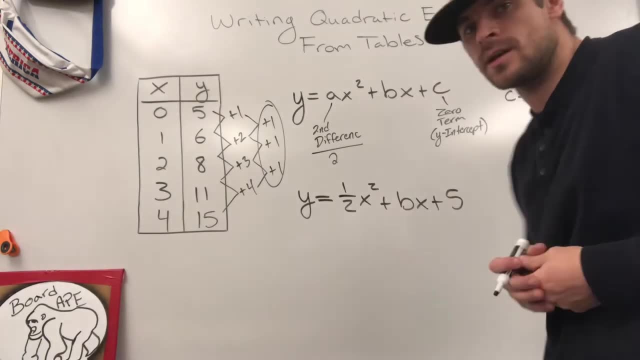 and plug in, Pick one and go with it. I recommend not using zero, okay, So I always use the one that's closest to zero, because those are typically the lowest numbers and small numbers are easy to work with. Come on, quit making your life hard. I got kids that will always choose four and 15,. 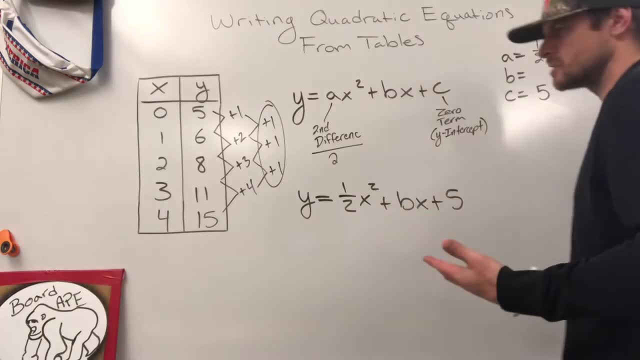 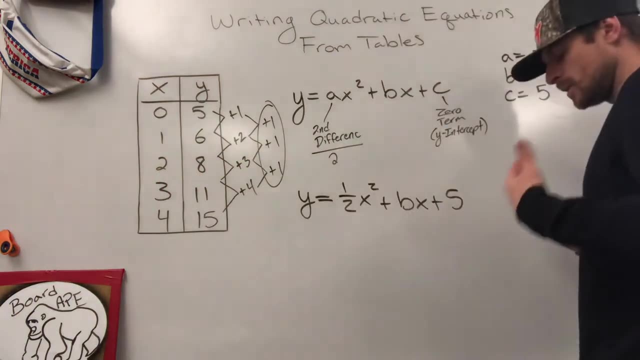 or these big numbers, and I'm like you're just making your life more challenging. Pick the easiest two numbers you can find. One and six look great. Two and eight look great. Now I will tell you one thing right now: If I'm going to take something and square it, 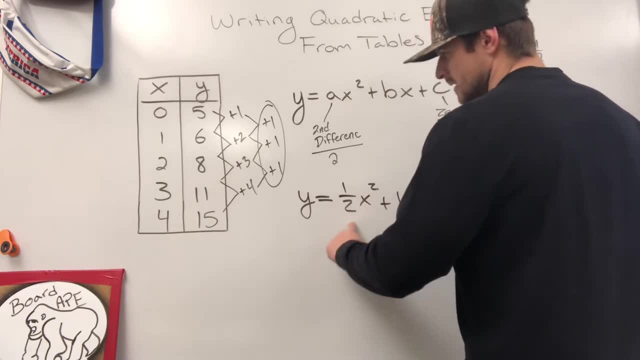 multiply it by a half. I'd like to get a whole number here. ideally, That means I need an. even If I put a one in and square it, I get one. and then multiply it by a half, I'm going to get a. 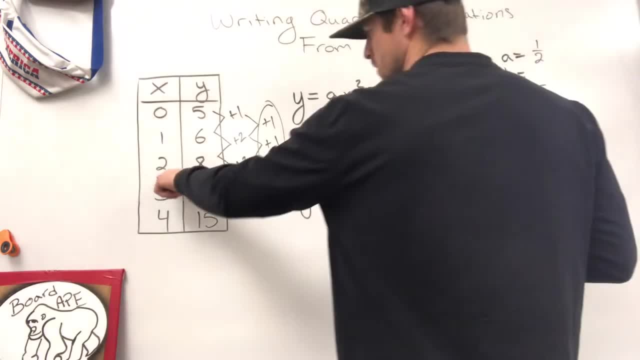 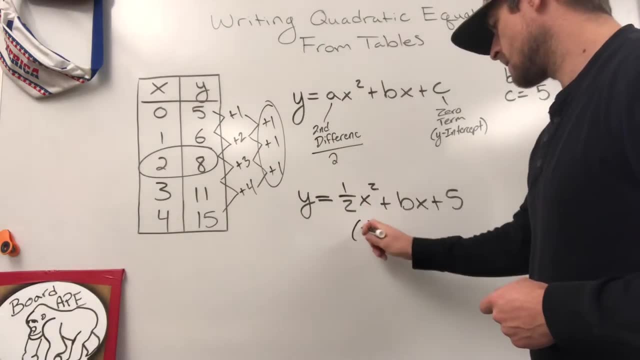 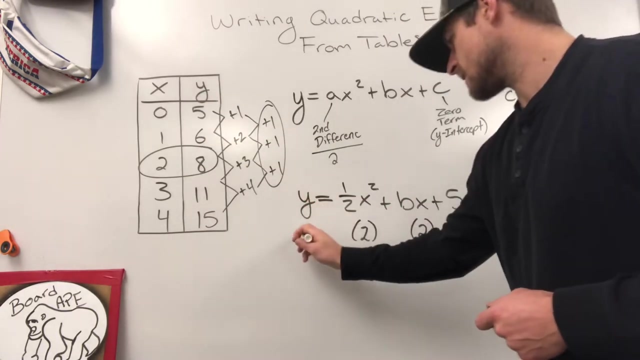 decimal 0.5.. I prefer not doing that, so I'm actually going to use two and eight. okay, Two is my x, so put a two wherever x is. Eight is my y, so put a eight where the y is. 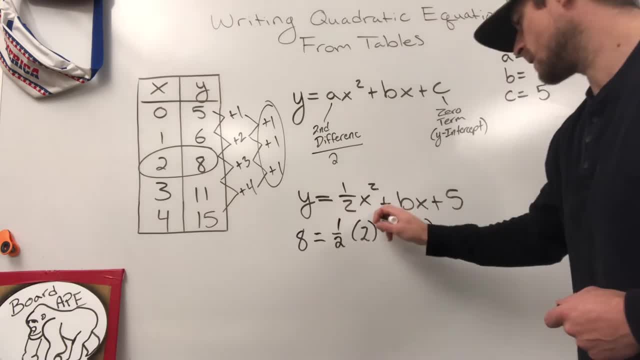 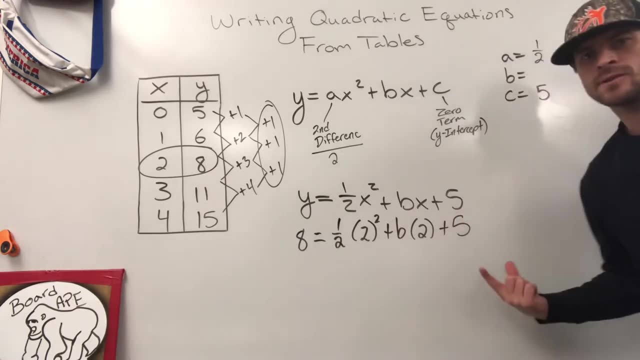 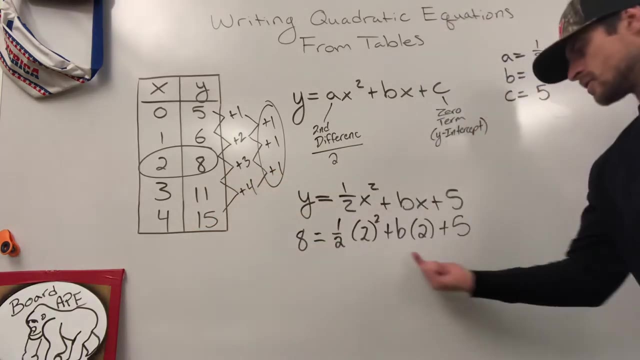 Everything else straight down. one half square it, b and plus five. So now what we have is we have an equation that we can simplify on the right side and then inverse operate everything over to the left so that b is isolated over here. All right, let's start doing it. Two squared is: 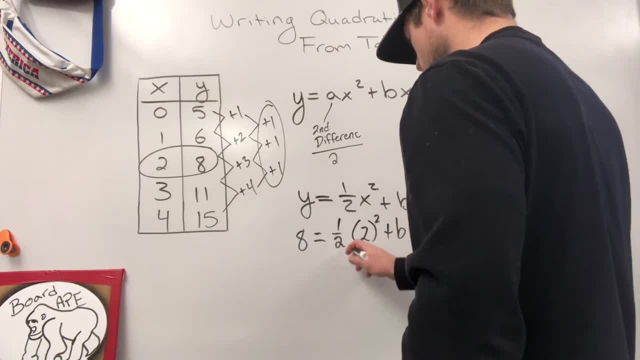 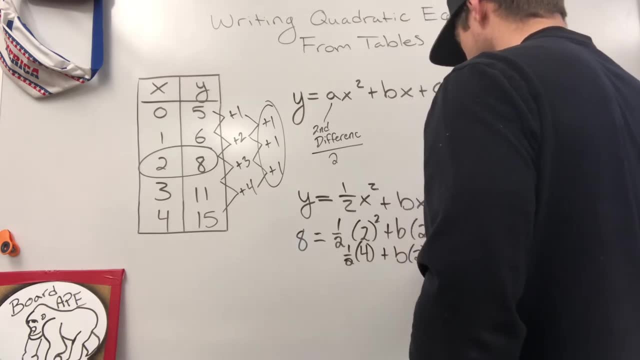 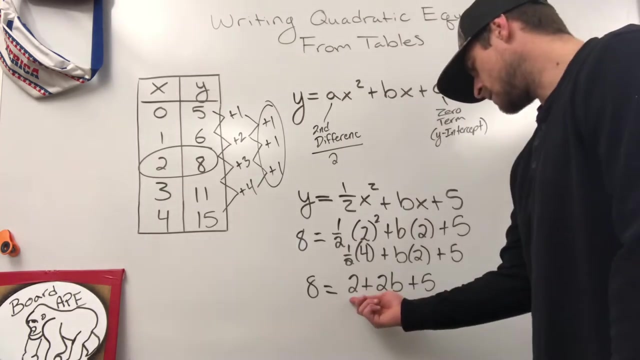 four, Four times one, half plus b times two plus five. Half of four is two plus. I'm just going to put that two in front as a coefficient to b plus five And remember it's equal to eight. All right, let's put the common. 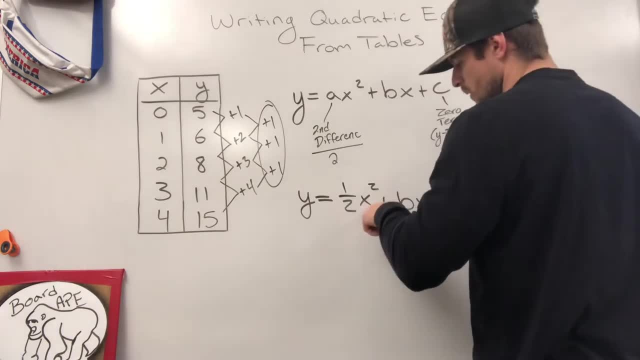 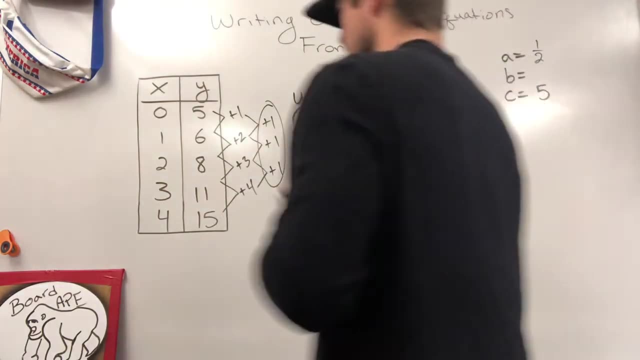 That means I need an. even If I put a 1 in And square it, I get one, And then multiply it by a half, I'm going to get a decimal 0.5.. I prefer not doing that, so I'm actually going to use 2 and 8.. 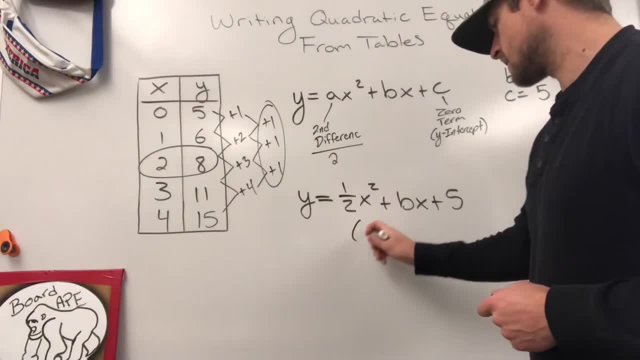 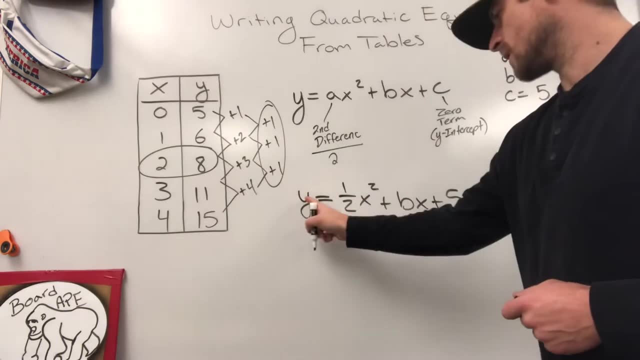 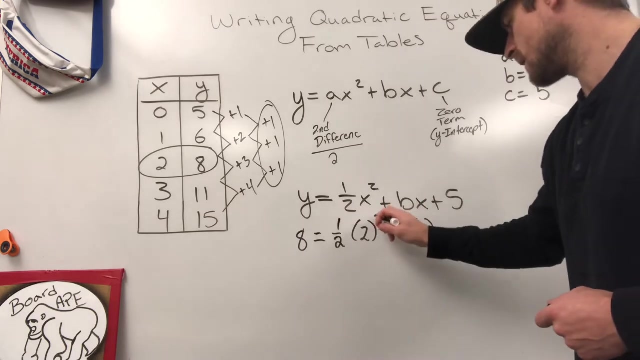 2 is my x, So put a 2 wherever x is. 8 is my y, So put a 8 where the y is. bring everything else straight down: 1, half square it, b and plus 5.. 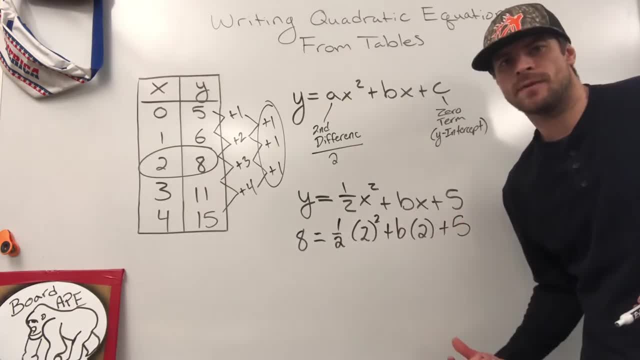 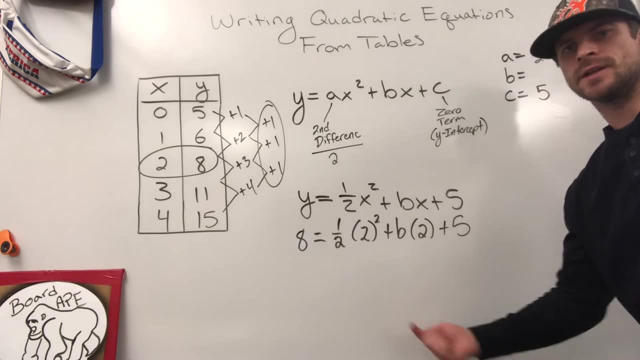 So now what we have is we have an equation that we can simplify on the right side and then inverse, operate everything over to the left so that b is isolated over here. All right, let's start doing it. 2 squared is 4.. 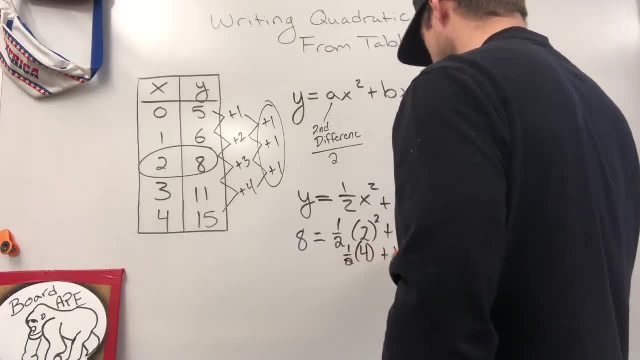 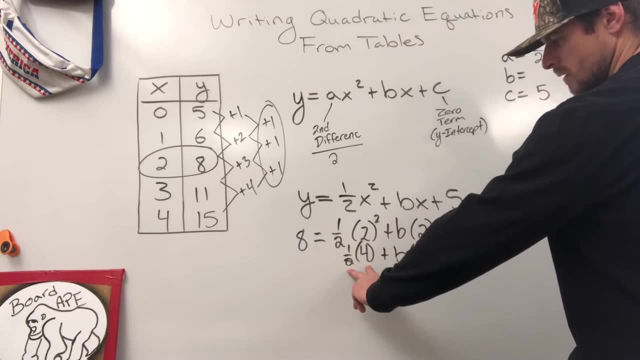 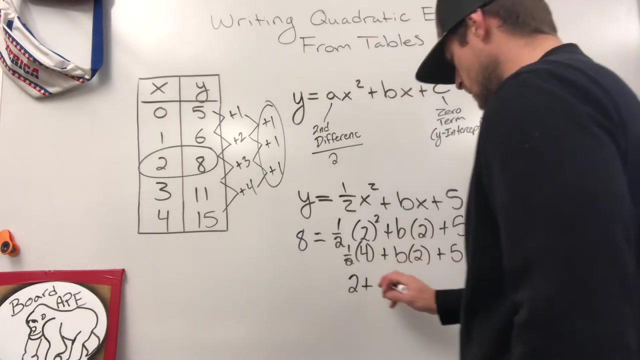 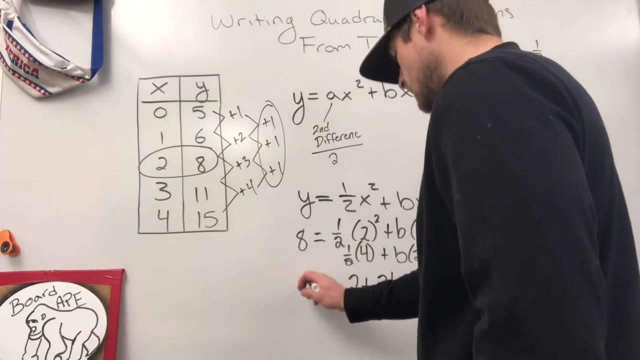 4 times 1, half Plus b times 2 plus 5.. Half of 4 is 2 plus. I'm just going to put that 2 in front as a coefficient: 2b plus 5. And remember it's equal to 8.. 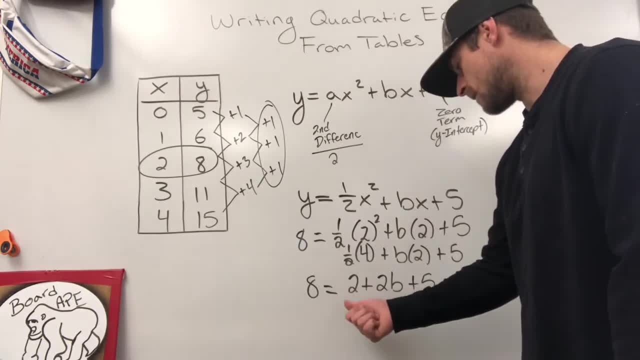 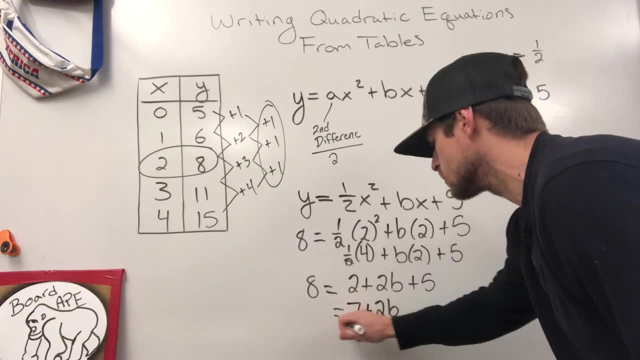 All right, let's put the common, or we're going to combine our like terms 2 and 5.. Put those together to make 7.. 7 plus 2b equals 8.. And because I'm running out of room right here, I'm just going to take this information. 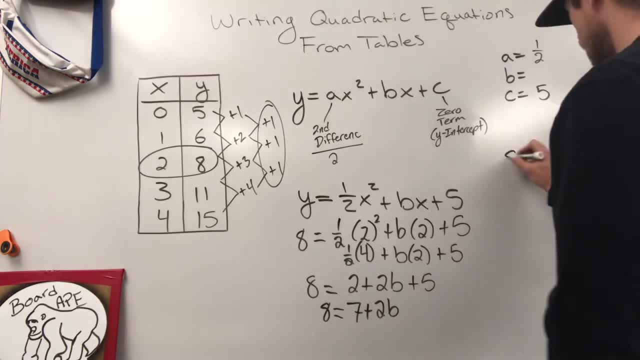 write it up over here and then you can finish working down. 8 equals 7 plus 2b. Take away the 7, cancels Take away the 7.. 8 minus 7 is 1.. 1 is equal to 2b. 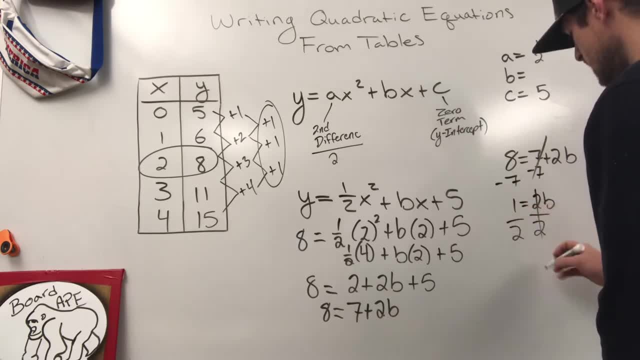 Divide by 2.. Divide by 2.. 2b is equal to 1.. So that's 1 over 2, or 1 half. Now I know what my b is And I know all 3 values that I need to write my equation out. 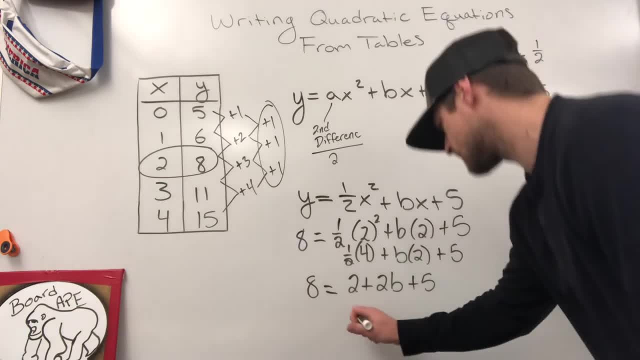 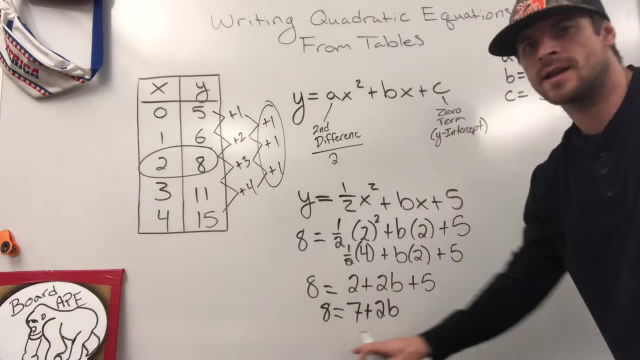 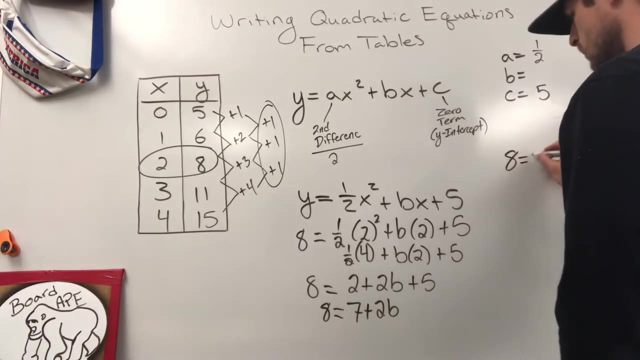 or we're going to combine our like terms: two and five. put those together to make seven. Seven plus two B equals eight, And because I'm running out of room right here, I'm just going to take this information, write it up over here and then you can finish working down. Eight equals seven. 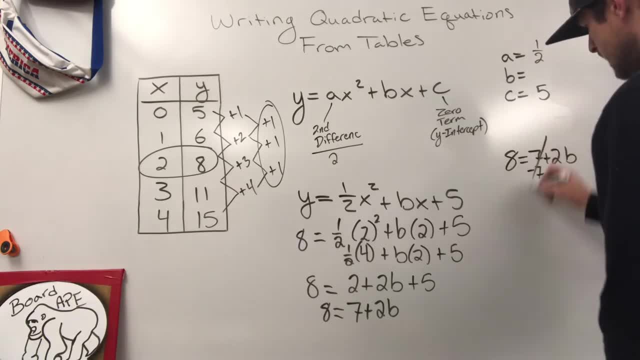 plus two b. Take away the seven. cancels. Take away the seven. Eight minus seven is one. One is equal to two b. Divide by two. divide by two B is equal to one over two or one half. 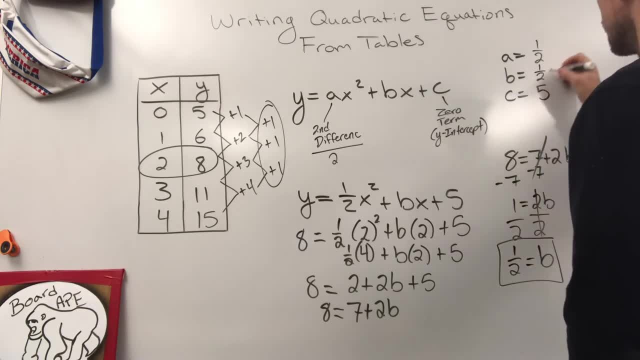 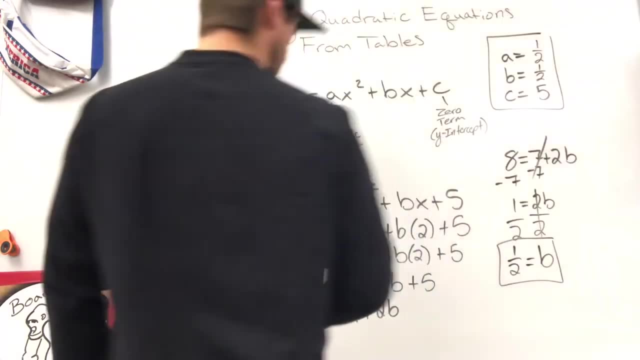 Now I know what my b is and I know all three values that I need to write my equation out. Okay, I'm going to write it right up here so you guys can see it nice and clear. I know my a. I know my. 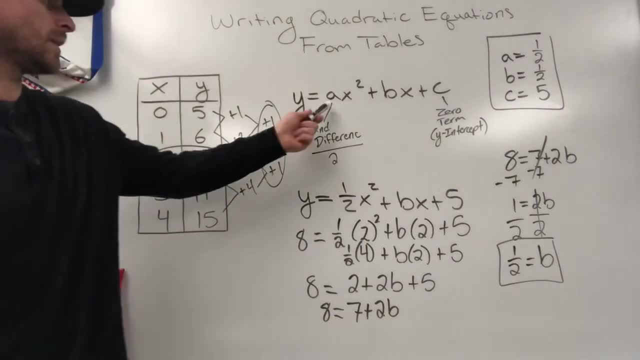 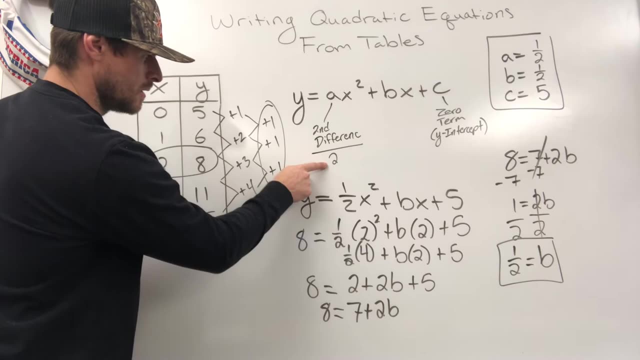 b. I know my c. Where did a come from? Well, it came from finding the first difference in the y column and then going out to the second difference and dividing it by two. That's the a. C comes from finding the zero in the n, finding the two, And I know that b is equal to one over two or one half. 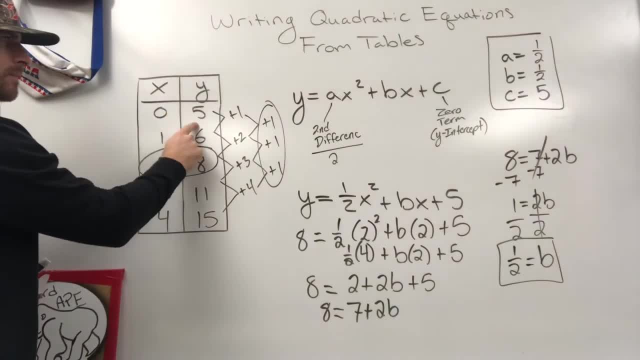 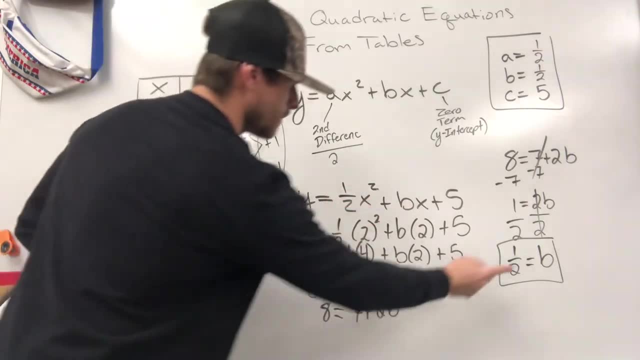 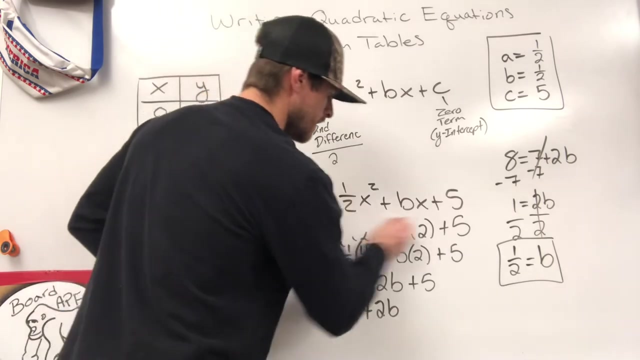 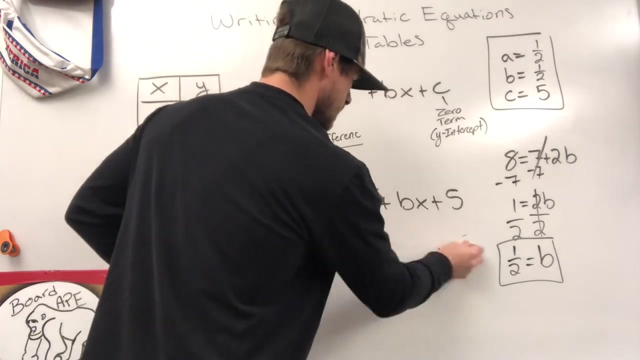 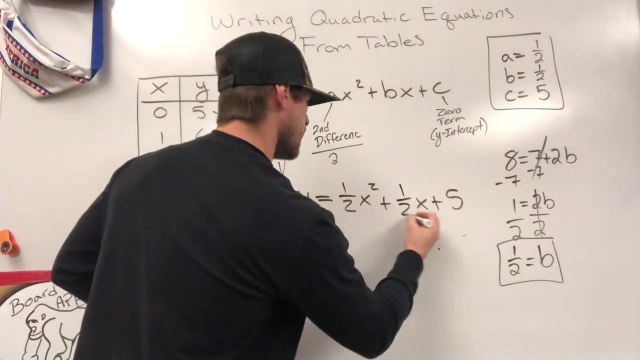 the table. it's the zero term, and then B. you plug everything that you know in, work it all out and isolate B to know what its value is. our final answer would be changing that B term right there to what we found it to be: 1 half X, Y equals. 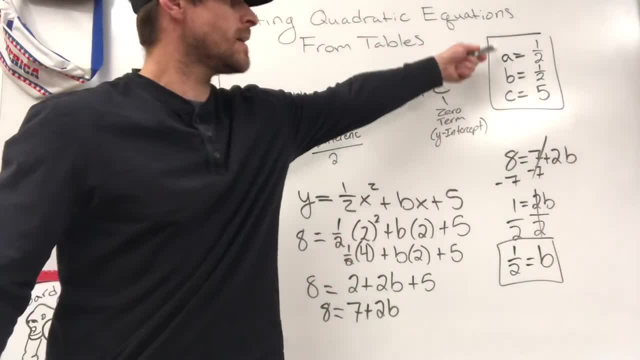 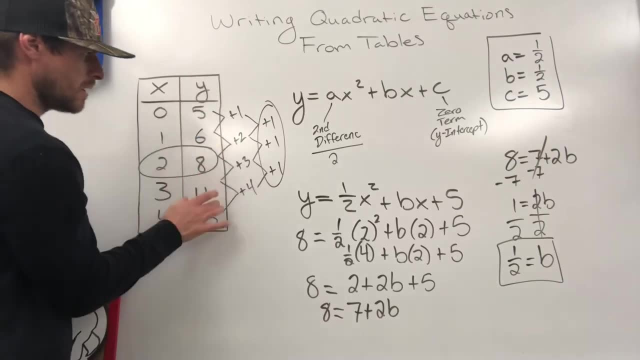 OK, I'm going to write it right up here so you guys can see it nice and clear. I know my a, I know my b, I know my c. Where did a come from? Well, it came from finding the first difference in the y column. 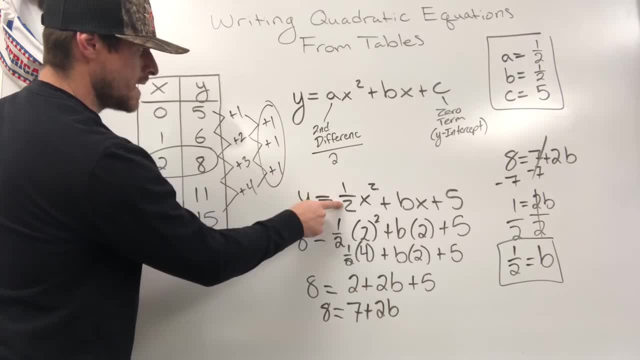 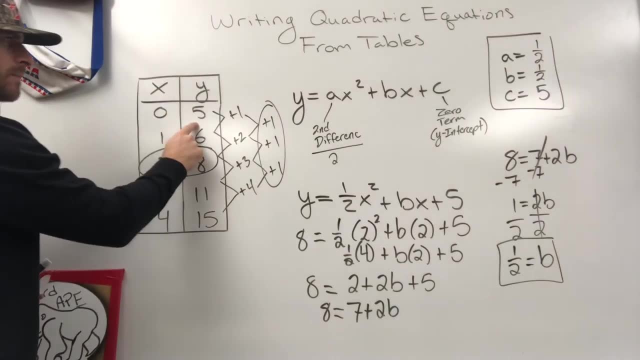 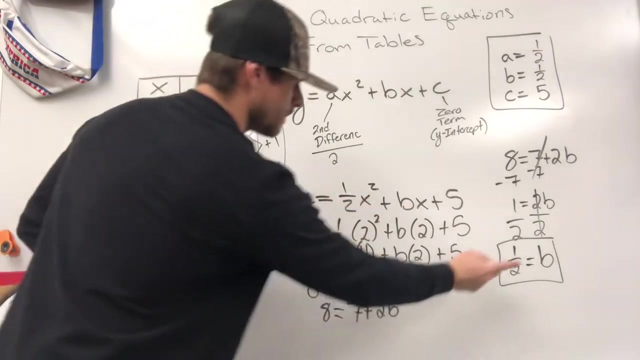 and then going out to the second difference and dividing it by 2.. That's the. a comes from finding the zero in the table, it's the zero term. and then B: you plug everything that you know in, work it all out and isolate B to know what its value. 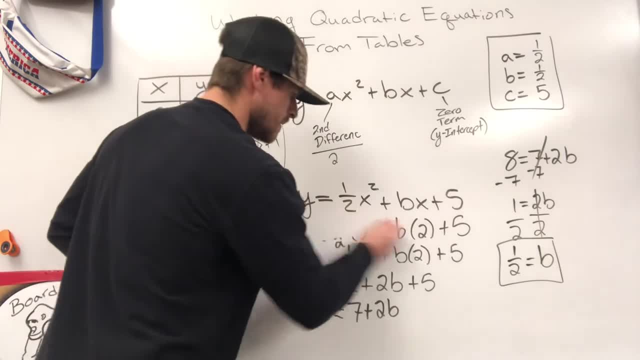 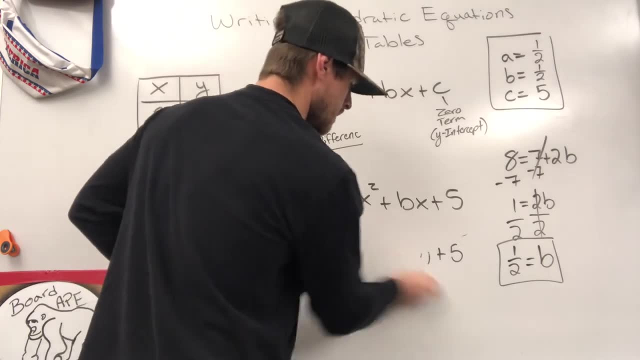 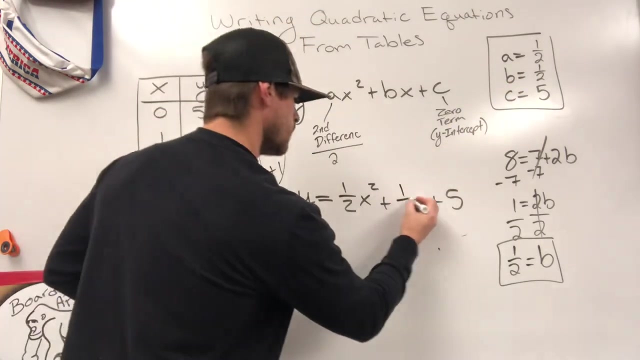 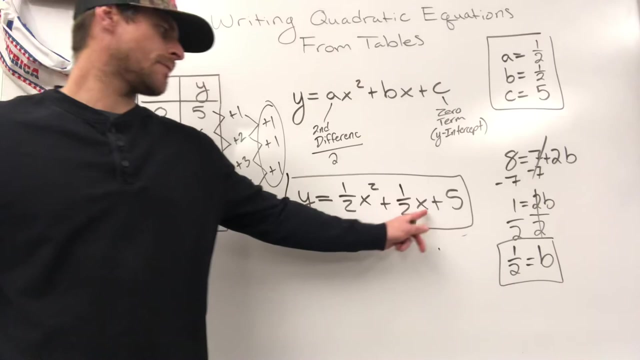 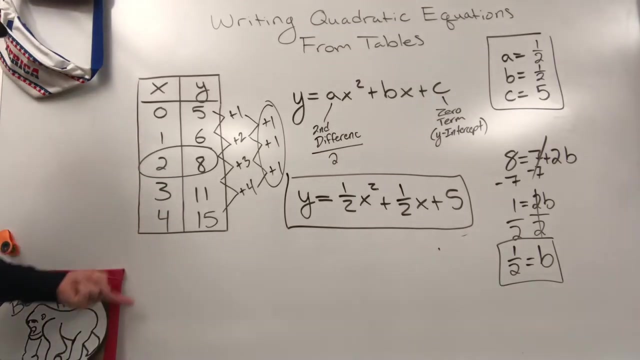 is. our final answer would be changing that B term right there to what we found it to be: 1 half X- Y equals 1 half X squared plus 1 half X plus 5. that quadratic equation would give you any value that you need. continued through this pattern, I can now throw a. 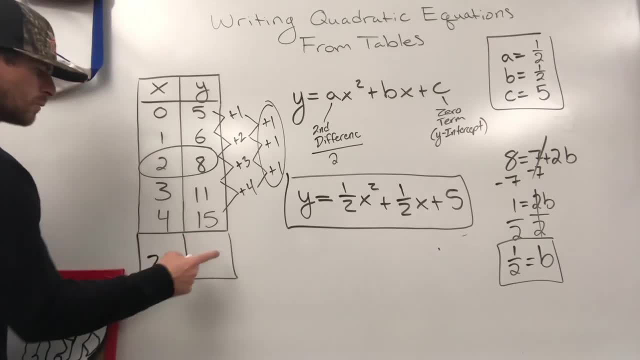 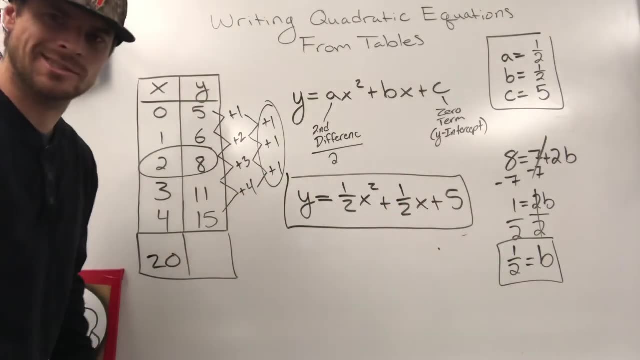 20 in there on a test and say what would Y be? you would put 20 here and here to determine what it is matter of fact. let's actually just go through with that, because you're probably going to be asked a question like that on your test. 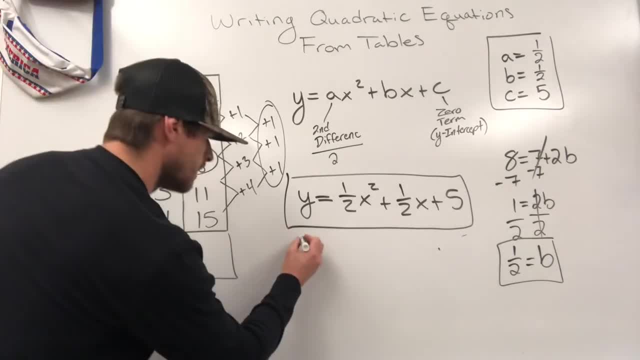 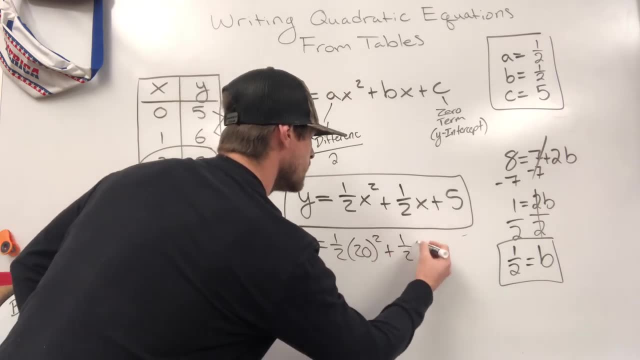 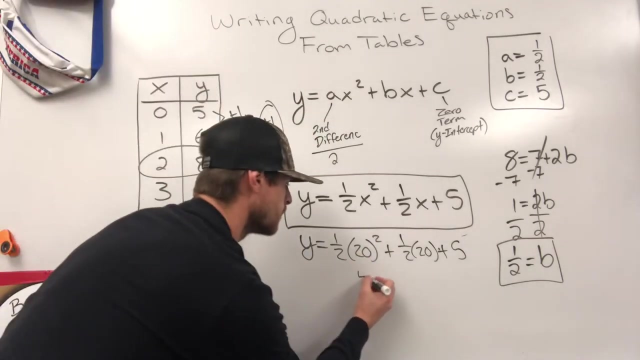 let's figure out what Y would be if X is 20. Y is equal to 1 half times 20 squared plus 1 half times 20 plus 5. 20 squared 20 times 20, it's going to be 400. we're going to cut that. 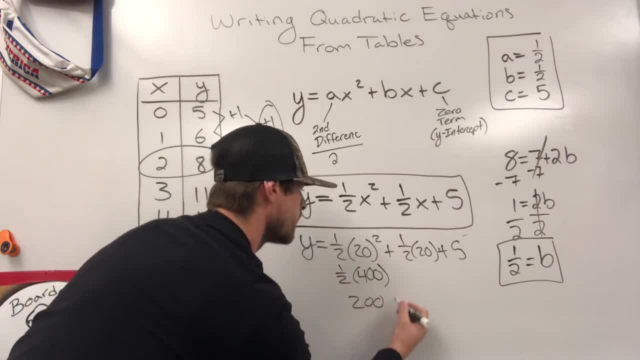 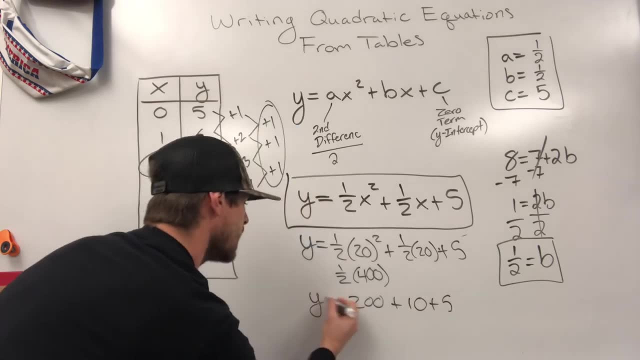 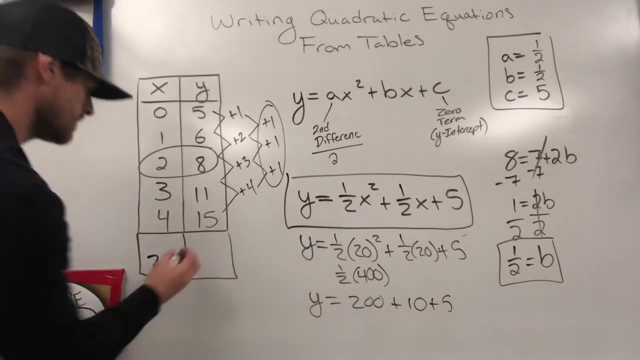 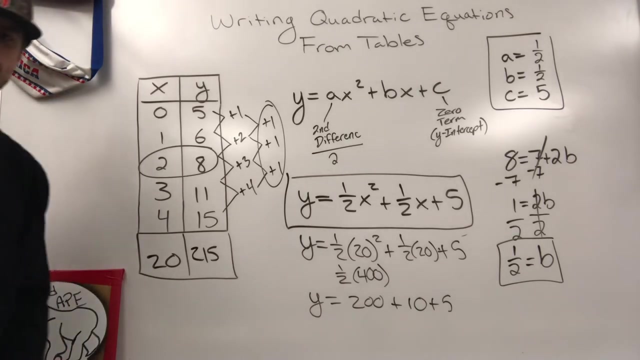 in half, which is going to give us 200 plus 1, half times 20. half of 20 is 10 plus 5, so Y is equal to 200 plus 1 plus 10 plus 5, 215. all right, hopefully this is making sense to you. study hard and good luck on your. upcoming test. 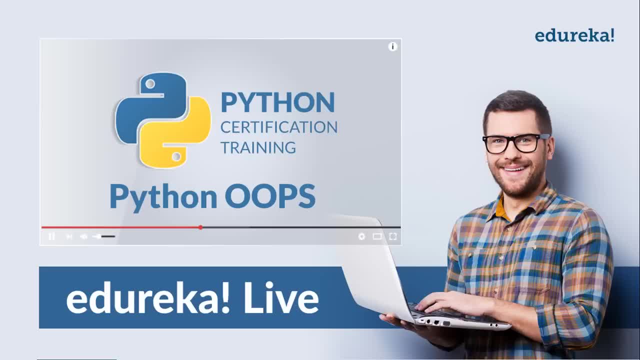 Hello everyone, this is Neil from Edureka and welcome to this Edureka live session on Python OOPS. OOPS, which basically stands for Object Oriented Programming System, or Object Oriented Programming as it's most popularly known, is one of the most popular programming. 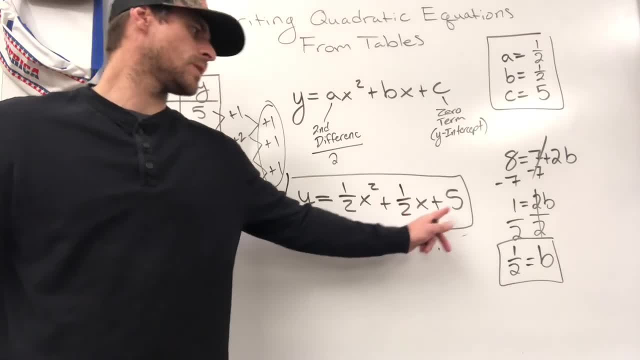 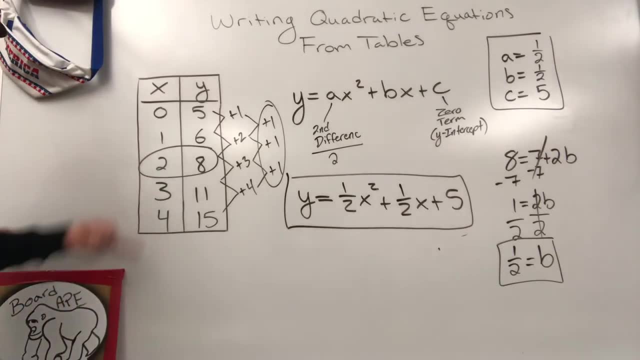 1 half X squared plus 1 half X plus 5, that quadratic equation would give you any value that you need. continued through this pattern. I can now throw a 20 in there on a test and say what would Y be? you would put 20 here and here to determine what it is matter. 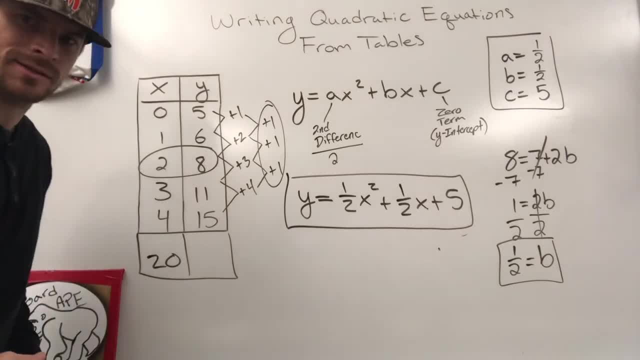 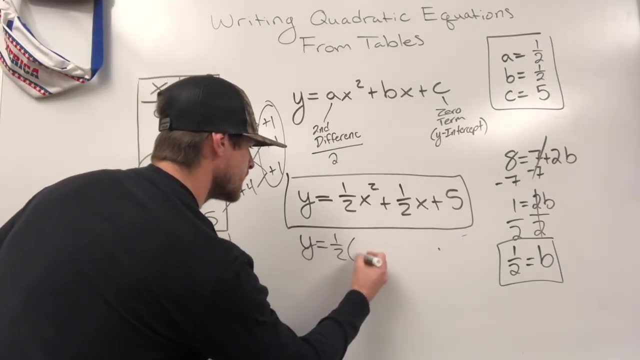 of fact, let's actually just go through with that, because you're probably going to be asked a question like that on your test. let's figure out what Y would be if X is 20. Y is equal to 1 half times 20 squared plus 1 half times 20 plus 5.